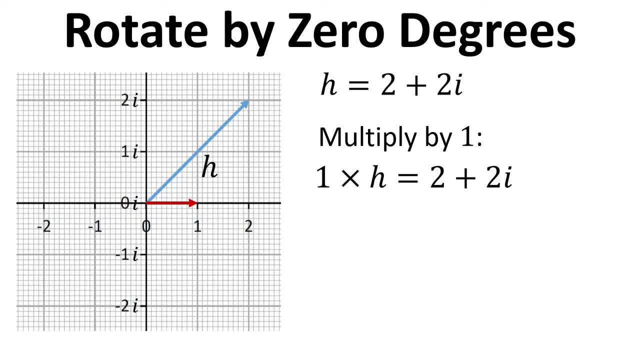 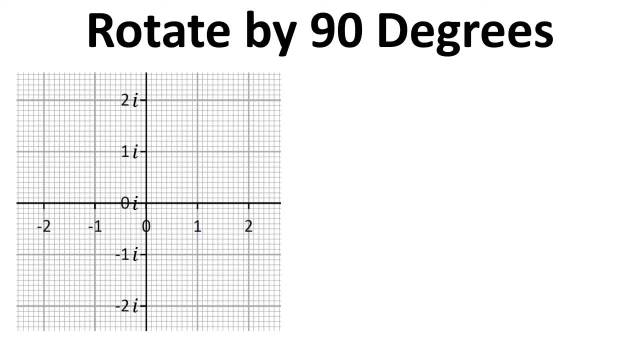 same complex number, and so the vector on the graph is completely unchanged. it just stays where it is Okay. but what about if we rotate by 90 degrees? To do this we need to multiply our vector by 1i. So we do 1i times H. that gives us i. 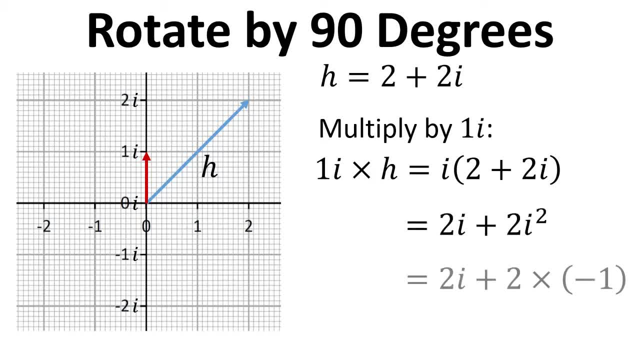 times brackets: 2 plus 2i. if we work that through, we end up with minus 2 plus 2i. If we plot that on, we can see that we've rotated by 90 degrees, and the reason for that is because 1i. 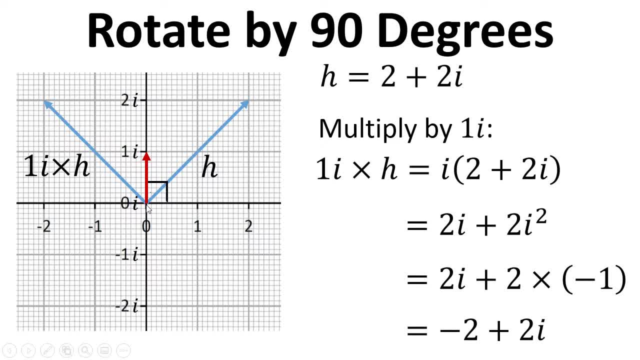 this red vector here is 90 degrees from the real axis. here where we have that original vector of 1 which rotated things by 0 degrees. So we've actually rotated anti-clockwise by 90 degrees and that's because this 1i is rotated by 90 degrees from from this. So the rotation of this vector has been. 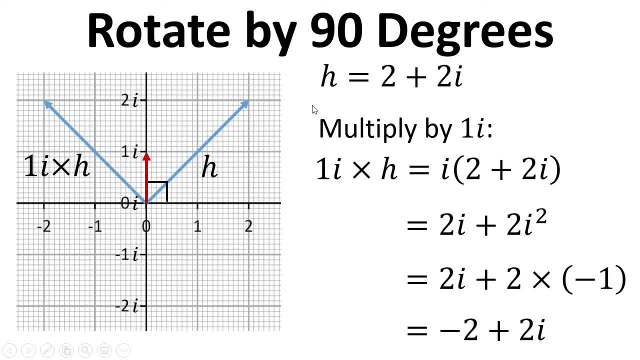 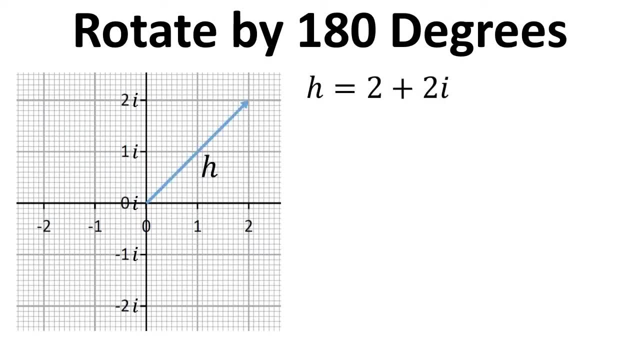 given to this vector, as it were, and because it's a magnitude of 1, it hasn't changed the magnitude of H. Okay, to rotate by 180 degrees we need to multiply by minus 1, so we can work this through. minus 1 times H gives us minus. 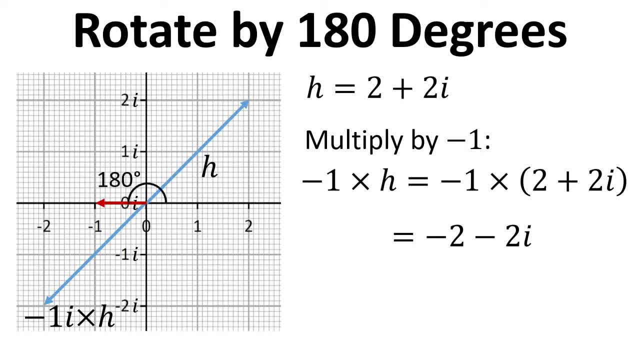 2 minus 2i, and now we've rotated by 180 degrees. And again, this is because this vector representing minus 1 is 180 degrees away from the vector that we had at the very start for just 1 on its own, positive 1.. Okay, and what about rotating by 270 degrees? Well, to achieve this, we 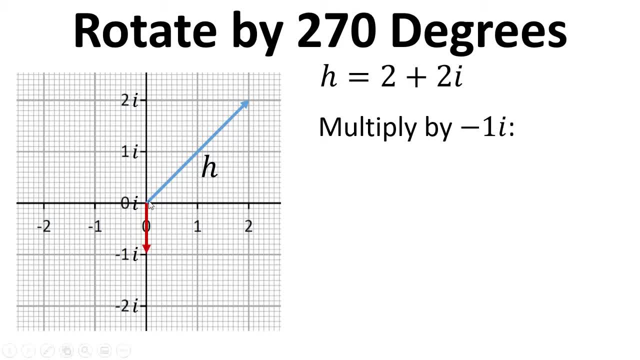 need to multiply by minus 1i so we can see: minus 1i is down here and if we multiply this through, we get minus 2i, minus 2i squared. Work this through and we get 2 minus 2i. and now that we can see, 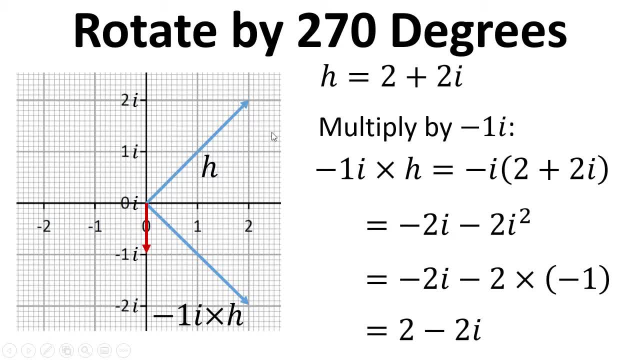 that this is rotated all the way around anti-clockwise, by 270 degrees And again, the explanation for this is that this vector for minus 1i is 270 degrees rotation away from when we have the vector for just positive 1 on the real. 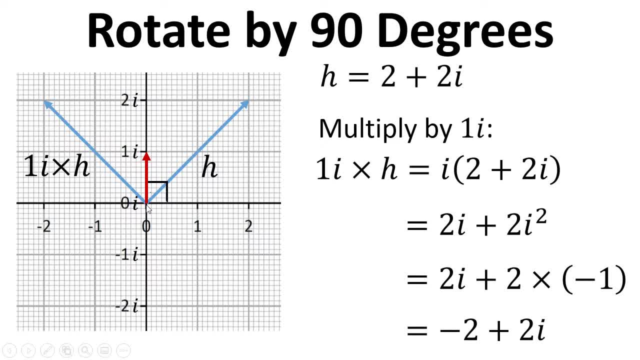 this red vector here is 90 degrees from the real axis. here where we have that original vector of 1 which rotated things by 0 degrees. So we've actually rotated anti-clockwise by 90 degrees and that's because this 1i is rotated by 90 degrees from from this. So the rotation of this vector has been. 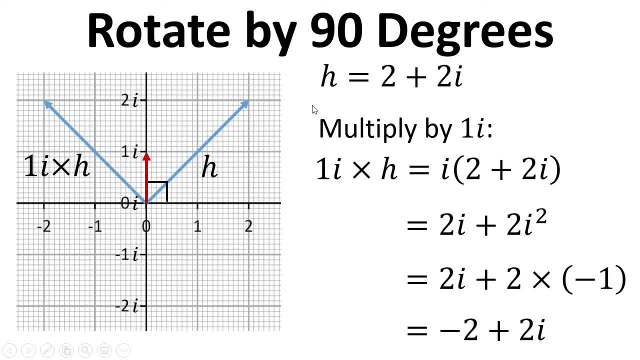 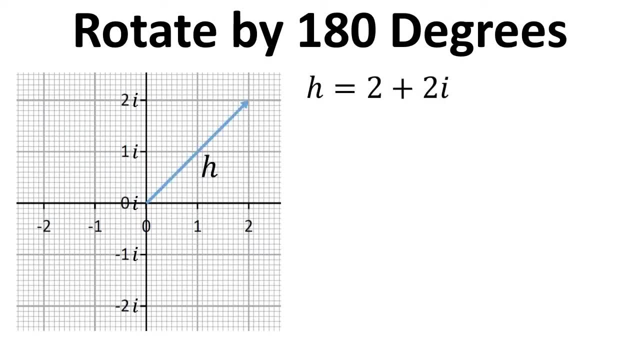 given to this vector, as it were, and because it's a magnitude of 1, it hasn't changed the magnitude of H. Okay, to rotate by 180 degrees we need to multiply by minus 1, so we can work this through. minus 1 times H gives us minus. 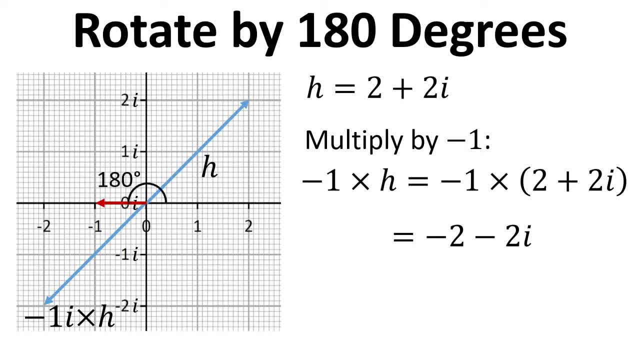 2 minus 2i, and now we've rotated by 180 degrees. And again, this is because this vector representing minus 1 is 180 degrees away from the vector that we had at the very start for just one on its own, positive 1.. Okay, and what about rotating by 270 degrees? Well, to achieve this, we 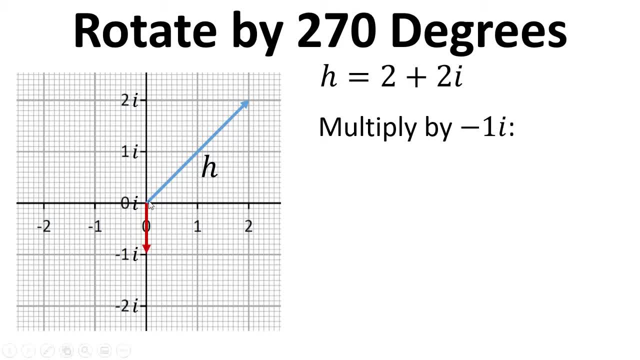 need to multiply by minus 1i so we can see: minus 1i is down here and if we multiply this through, we get minus 2i, minus 2i squared. Work this through and we get 2 minus 2i. and now that we can see, 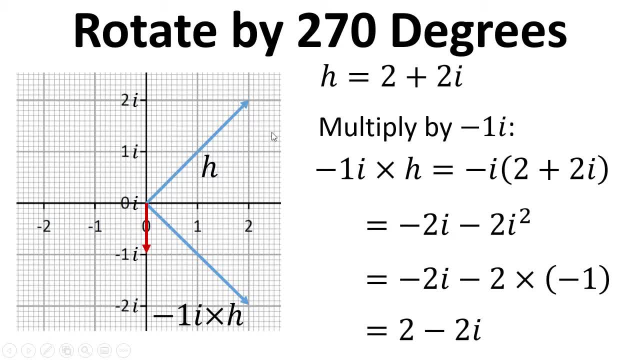 that this is rotated all the way around anti-clockwise, by 270 degrees And again, the explanation for this is that this vector for minus 1i is 270 degrees rotation away from when we have the vector for just positive 1 on the real. 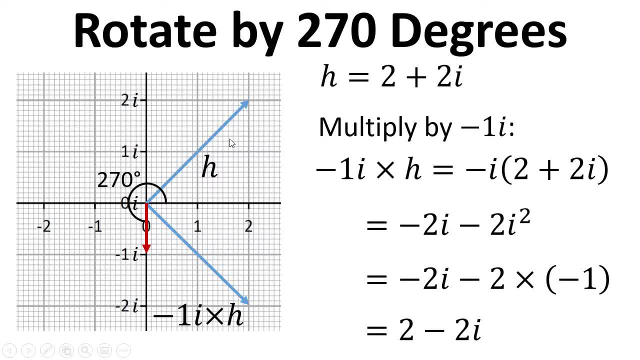 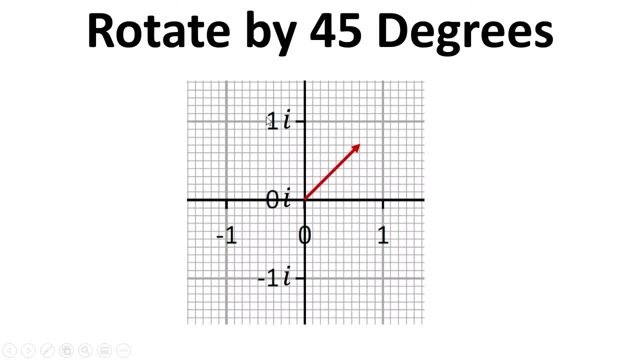 axis here. So we can rotate our vector. and as long as the magnitude of the thing we're multiplying by the vector that we're multiplying by is 1, we won't change the size, we'll just give it the rotation from that vector. So what about if we wanted to rotate by 45 degrees? We'd need 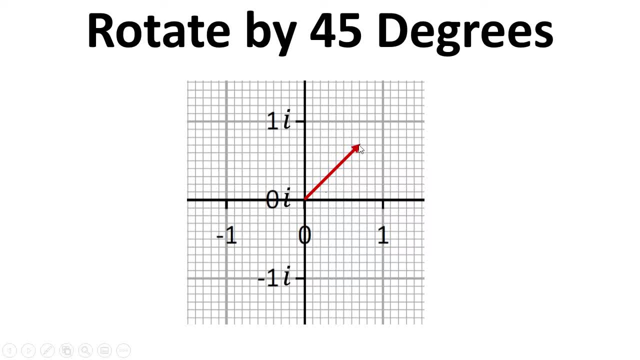 a vector magnitude 1, so that it wouldn't change the magnitude of the vector we're multiplying by, and we'd need it to have a 45 degree angle from the real number line here. So how big would the real part need to be and how big would the imaginary part need to be? I'm going